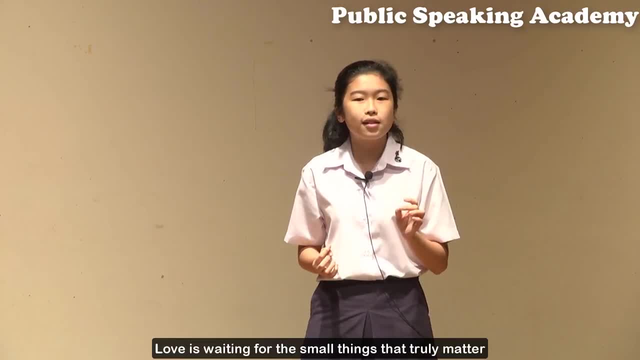 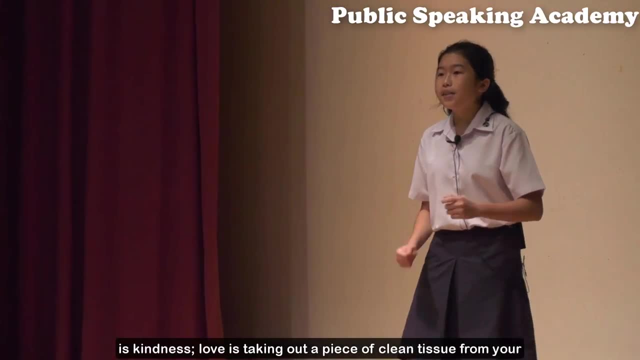 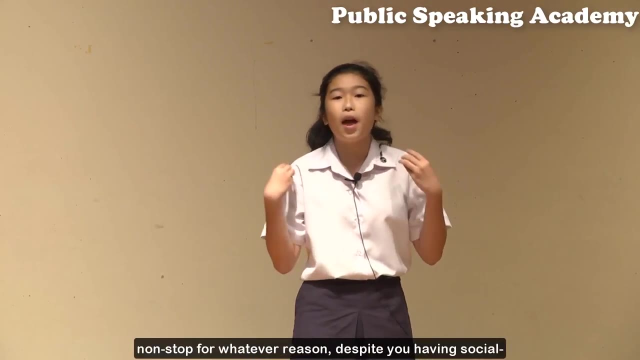 you love her. love is waiting for the small things that truly matter. even if you are naturally impatient, love is kindness. love is taking out a piece of clean tissue from your bag, offering it to a lady who has been crying on the bus non-stop for whatever reason, despite you having social anxiety, and you find it so. 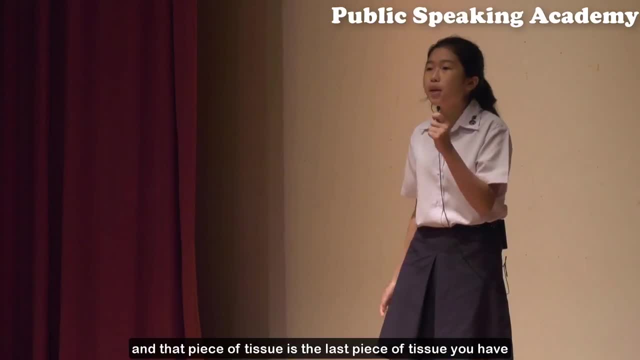 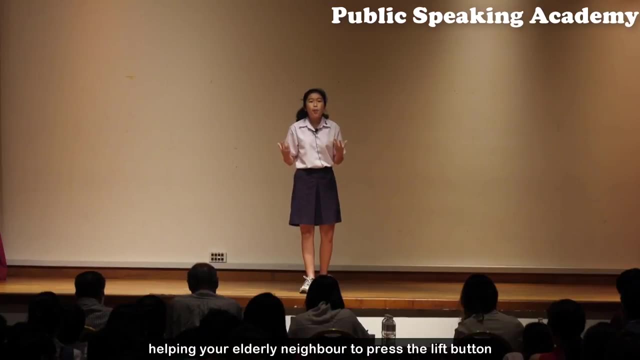 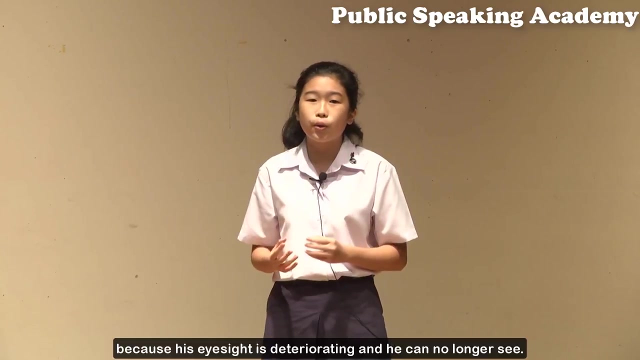 hard to talk to others. you give it to her and that piece of tissue is the last piece of tissue you have in your bag for the rest of the day. love is helping your lift your elderly neighbor to press the lift button because his eyesight is deteriorating and he can no longer see. you do this for him every time he comes. 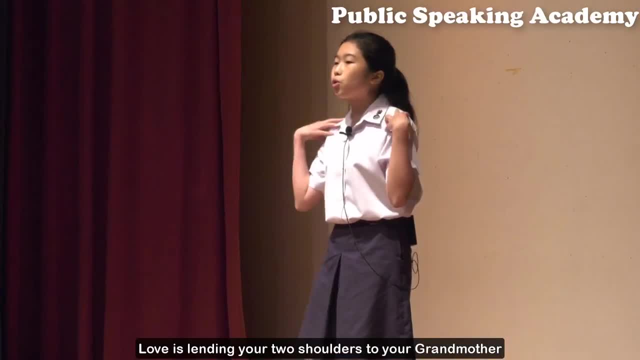 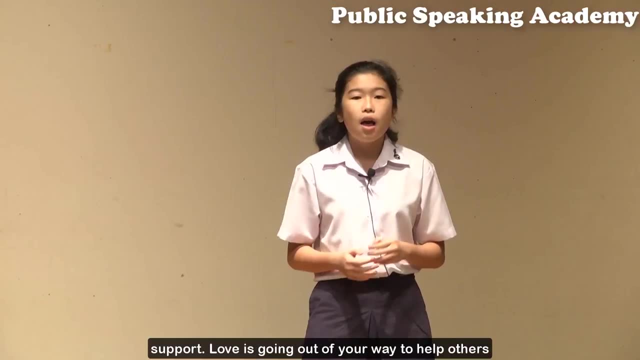 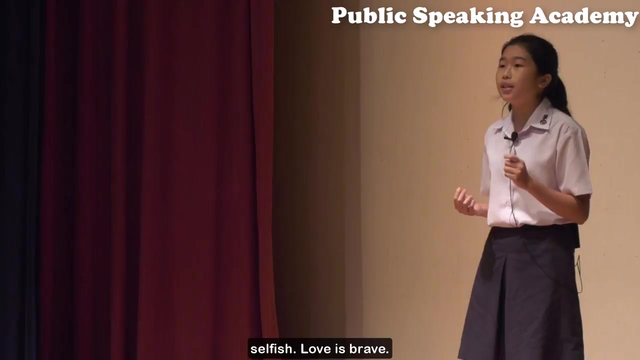 into the lift. love is lending your two shoulders to your grandmother. can no longer balance on her two feet and now lean on you for support. love is going out of your way to help others around you, people that you love, despite you being naturally selfish. love is brave. love is. 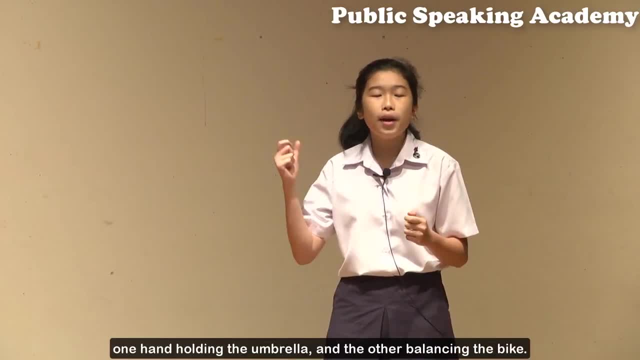 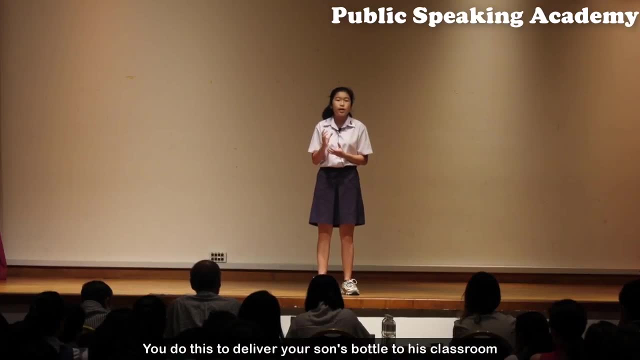 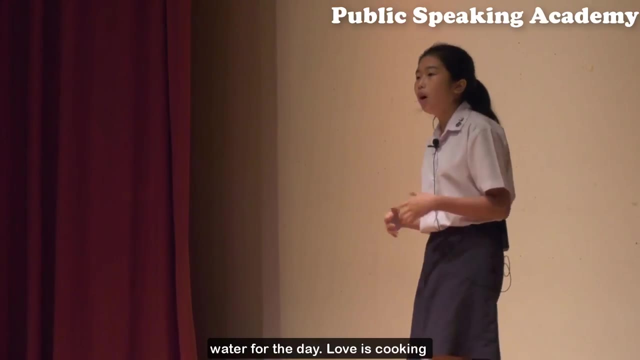 cycling in the rain, braving the storm, with one hand holding the umbrella and the other balancing the bike. you do this to deliver your son's bottle to his classroom, because he left it at home, because you want him to get enough water for the day. love is cooking porridge for your sister who is so sick, weak and tired to get up. 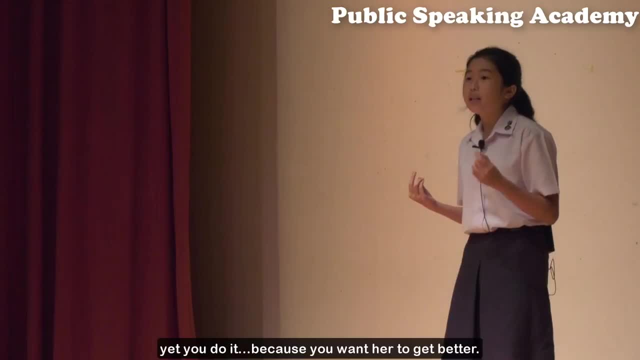 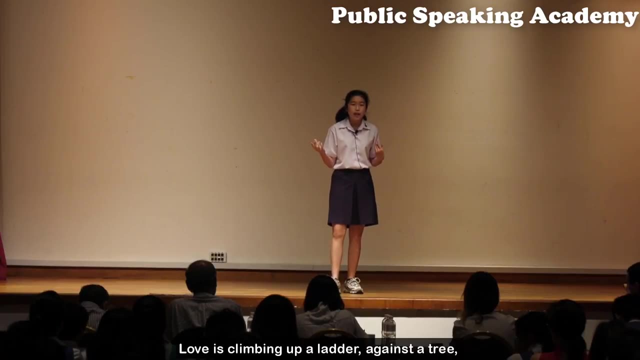 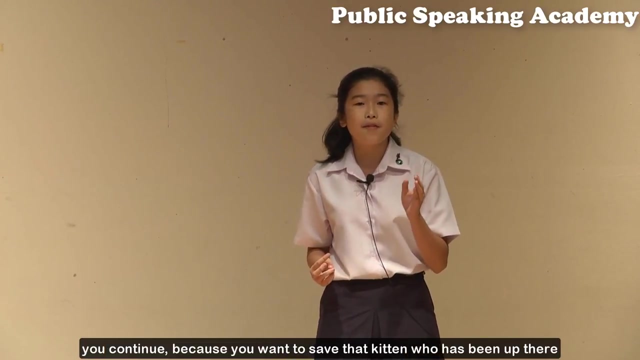 from her bed. you are so scared of the fire, yet you do it because you want her to get better. love is climbing up a ladder against a tree, constantly peeping down, because you are so scared of falling, but you continue because you want to save that kitten who has been up there for hours. 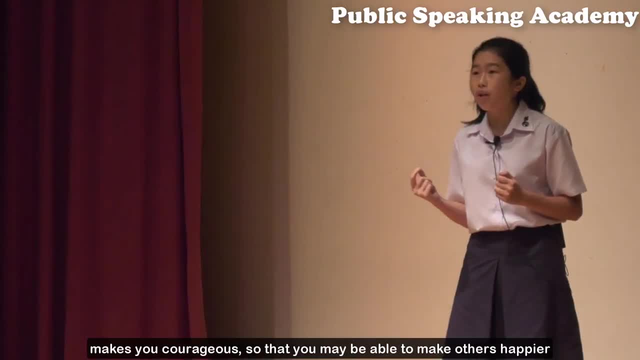 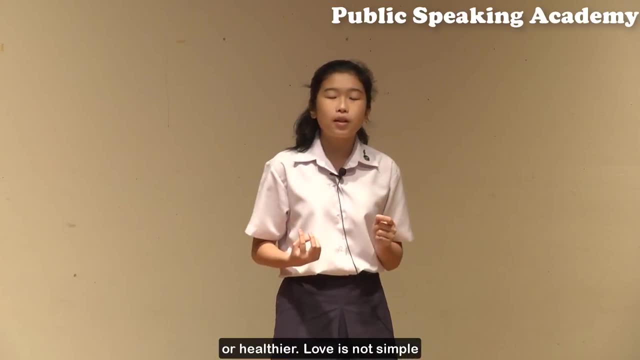 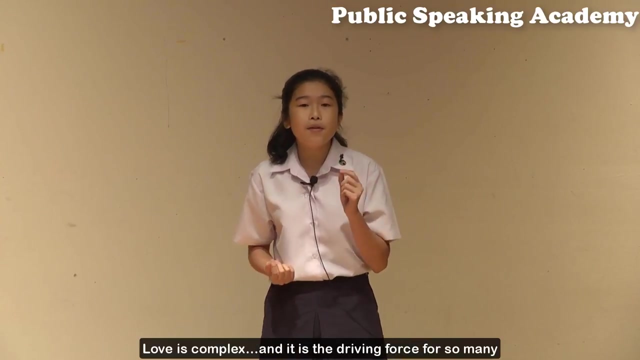 love makes you do the bravest things, makes you courageous so that you may be able to make others happier or healthier. love is not simple and it is not just sweet but empty words. love is complex and it is the driving force for so many wonderful virtues. love is what makes an 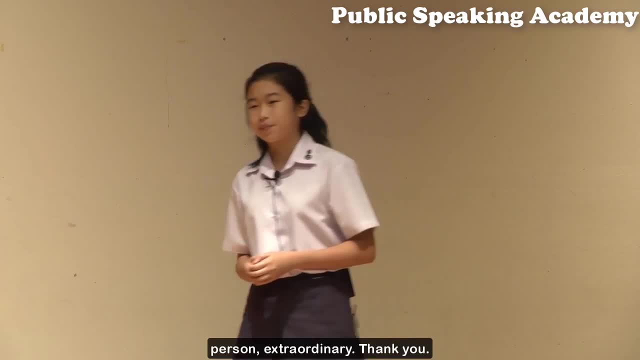 ordinary person, extraordinary. thank you.